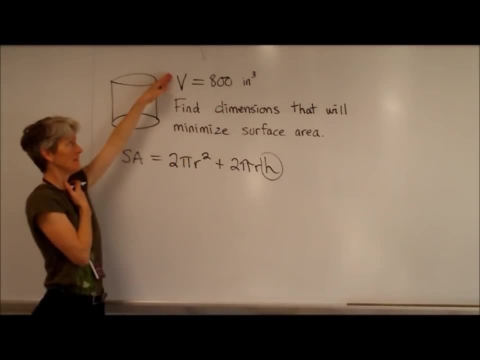 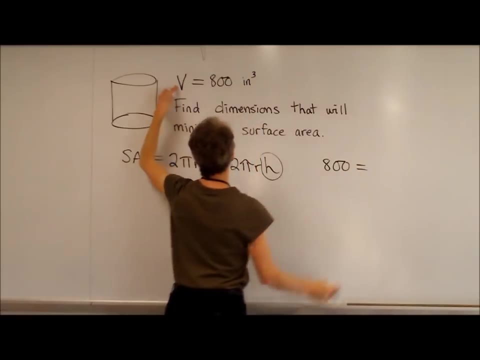 to the given information and see what I haven't used yet. And I know something about the volume. So my volume is 800 cubic inches. Huh, I know the volume of the cylinder. What's the volume of the cylinder, Mr Haas? 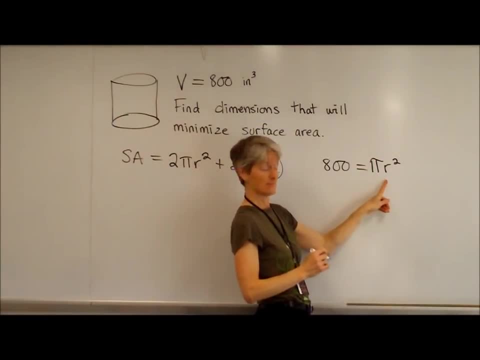 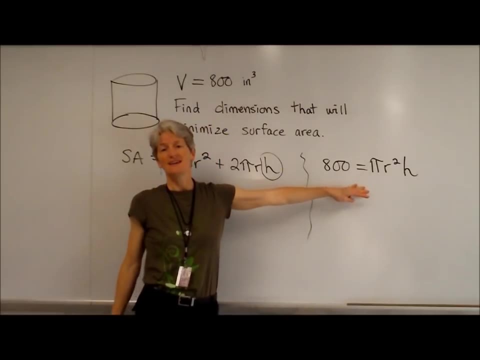 Well, it's just the area of the bottom, the area of the base, which is a circle, very nice area of a circle, times how tall it is, which I guess you're calling h, Very nice. This will give me a very handy expression for h that I can then substitute. 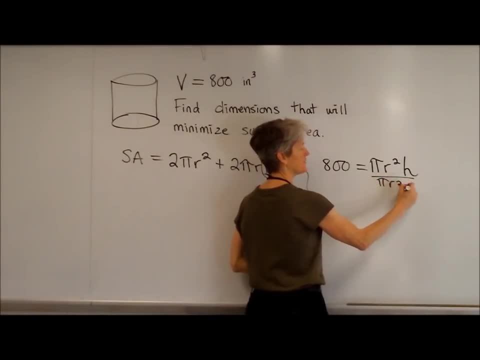 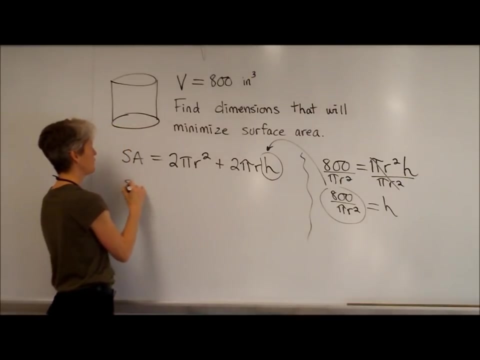 in here. So here I go. I'm just going to divide by pi r squared. So h is equal to 800 divided by pi r squared. And in I go, Boom. So surface area: 2 pi r squared plus 2 pi r squared. So 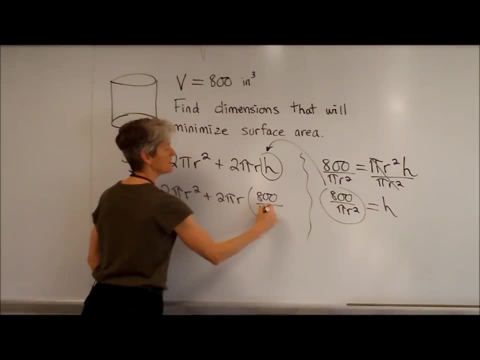 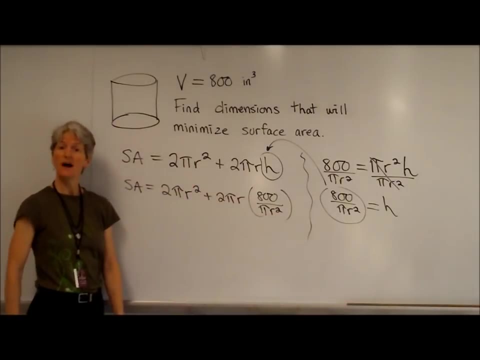 r times that whole business. Now I have my equation for service area, just in terms of r. Let's clean that up though, shall we? What do you think Sounds good? I can throw that over 1.. I can do some dividing before I multiply. 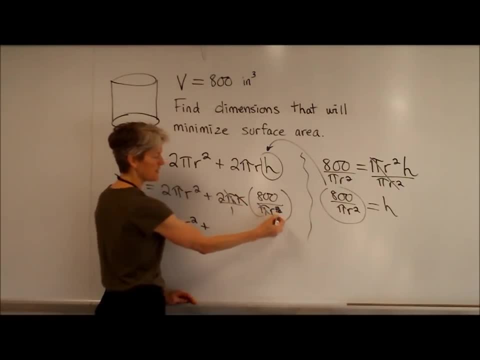 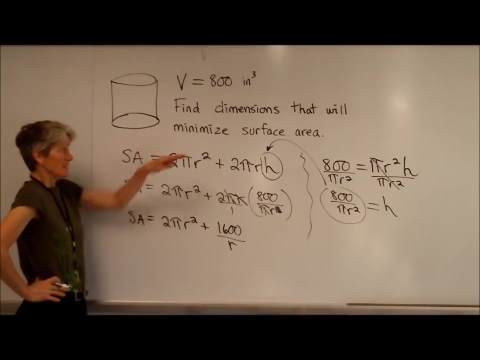 Pi divided by pi is 1.. r divided by one of those r's is 1.. So it looks like I have 2 times 800, which is 1,600 in the numerator, 1 times r in the denominator. So, as I think you know by now, what I want to do is to find a minimum surface area. 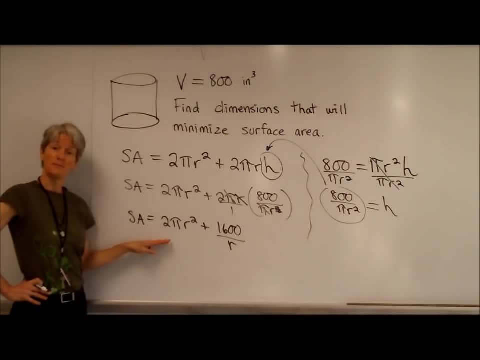 I want to find a point where this has a minimum To do that. I want to find the slope. To find the slope, I take the first derivative And we know that at a minimum, the first derivative is 0.. The slope is 0.. 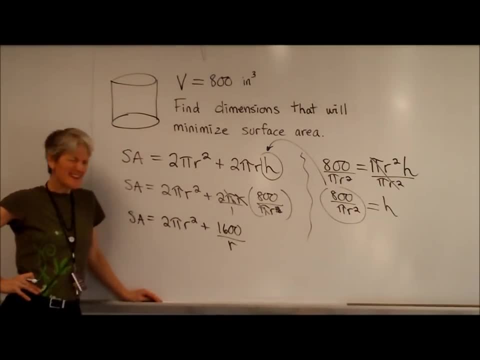 So let's take the derivative of this. You know, I think I want to rewrite it before I take the derivative, because I don't want to do the quotient. Oh yeah, You want to bring that r upstairs? Yeah, absolutely. 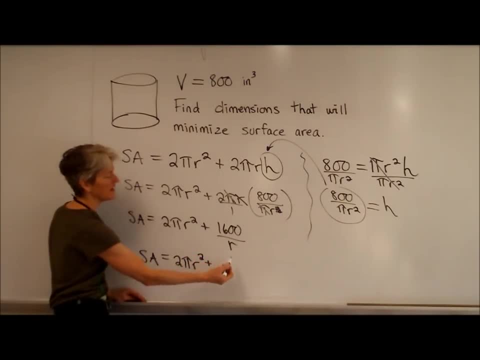 Bring that r up into the numerator Again. I think we're getting good at this. now. Move that up, which means I'm going to call it r to the negative 1.. So far, so good, Sounds good. Is that why we do a lot of algebra practice? so they can like move. 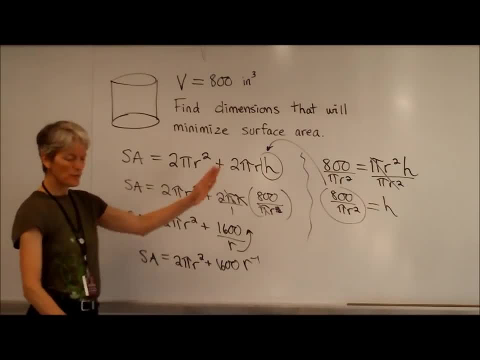 I know, All right, I know It's really, it's great. Okay, I'm going to move over here. I'm just going to erase this bit because I think we're probably good Give myself a little more room. 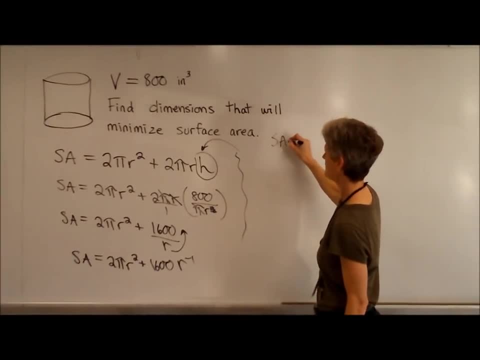 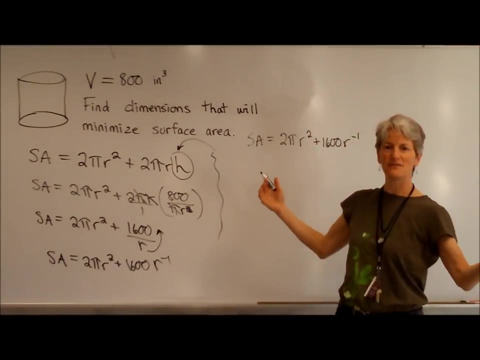 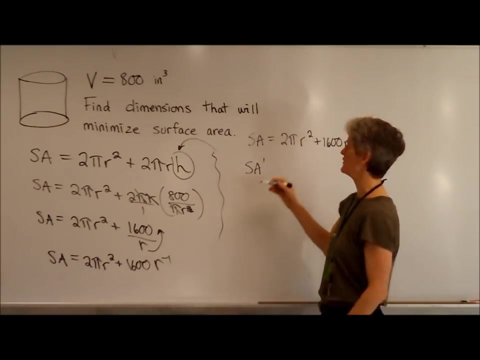 So I've got my surface area 2 pi r squared, plus 1600 r to the negative 1, taking the derivative, The derivative of surface area is just the derivative of surface area. I hope that's all right. I'm using two variables there. 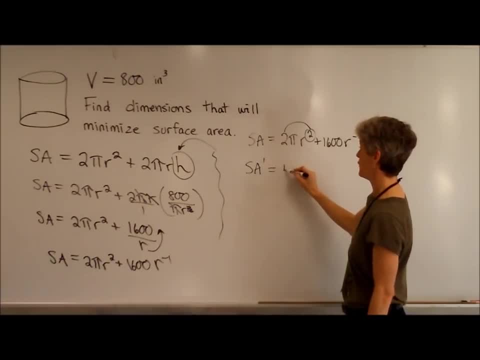 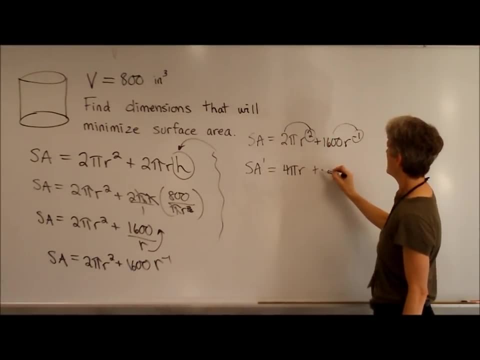 Okay, here we go. 2 times 2, pi is just 4 pi r. Remember, pi is just a number Negative 1 times 1600.. Oh, let's just call that minus 1600 r to the negative 2.. 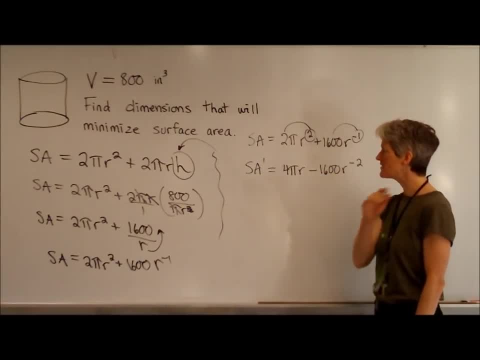 That's my slope, my first derivative. I want to find when the slope or the first derivative is equal to 0, or where it's undefined. So at this point I'm now going to rewrite this with that r squared in the denominator. 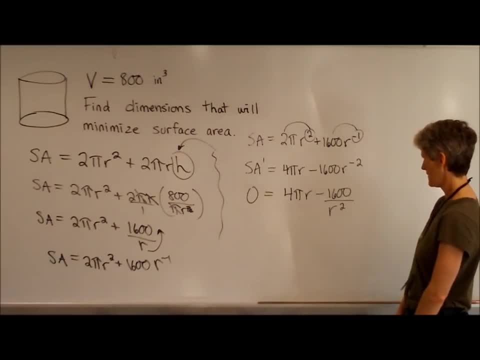 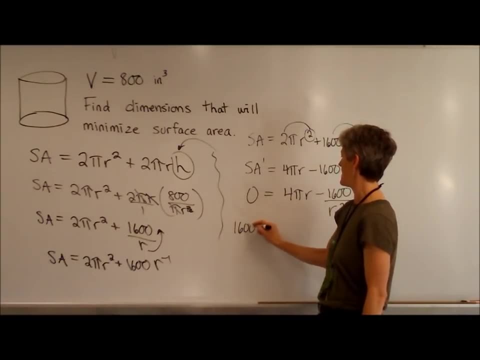 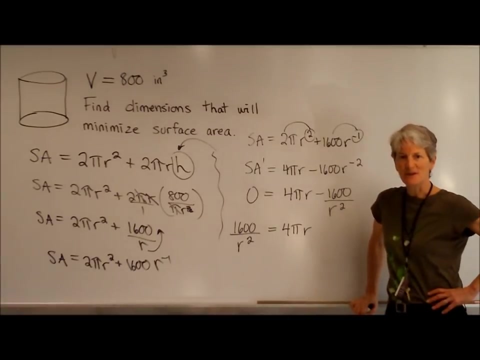 Just because it's easier for me to see what's going on. I'm solving for r, So let's see, I think I'm going to move this over here. add that term to both sides. Wow, this is looking a little complicated, Mr Haas. 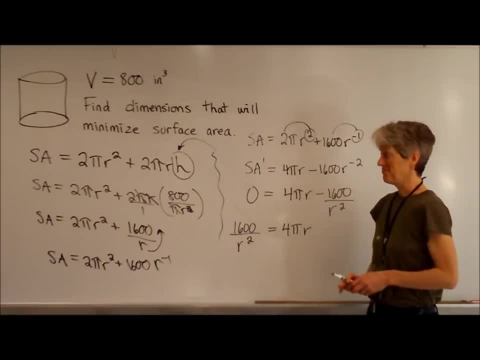 Any ideas what I should do? I think you could multiply both sides by r squared. That sounds good. Yeah, whenever we have a fraction, you can always get rid of the fraction by just multiplying both sides. Okay, Multiplying both sides by that denominator. 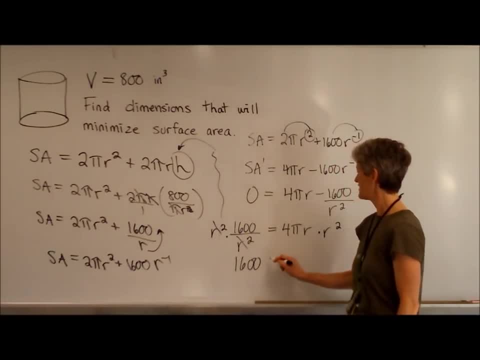 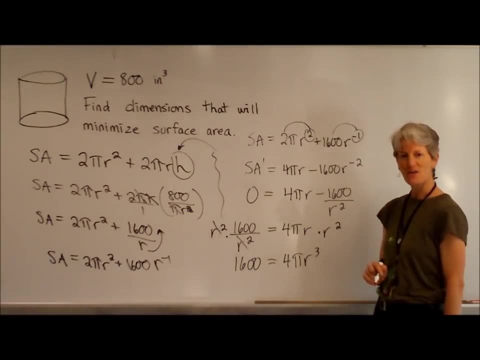 Goodbye denominator. Here we have 1600, 4 pi. r to the 3rd. Don't be intimidated by that r to the 3rd, We can handle that. Let's get it by itself. Let's divide by 4 pi. 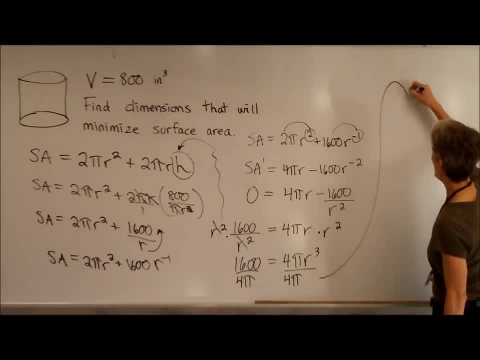 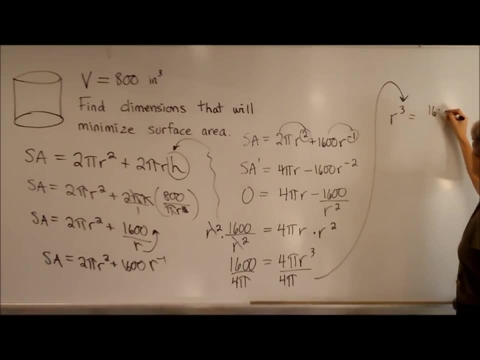 This is getting good And I need more room. Oh, can you see me up here? Yeah, I got you. Okay. So I have r cubed equals 1600 divided by 4 pi. How do I get that r by itself? 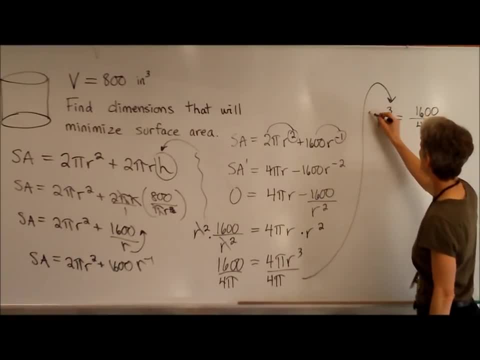 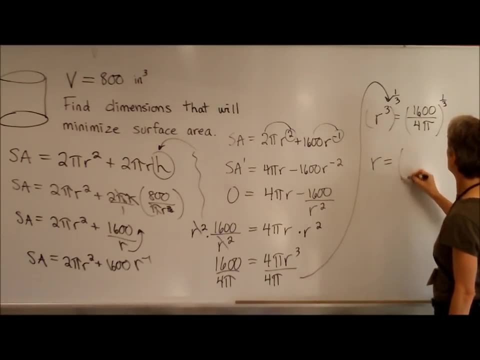 I think you're going to have to take the cubed root. You're very good at this. Yeah, thanks, Let's take the cubed root. I'm just going to write that as raised to the 1- 3rd, And that is something that we can. 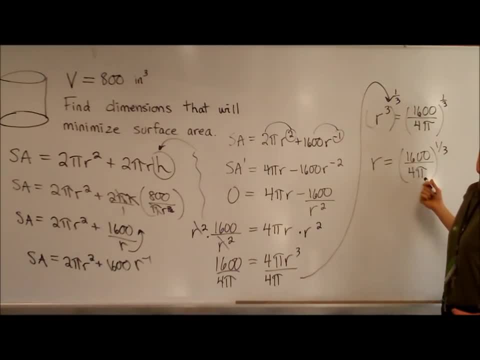 I mean, that's exact form, like that. But we can figure out what that is in decimal form By throwing that into your calculator, And I think I have a student here who's going to help me calculate this. Fantastic, Do you have a calculator with you? 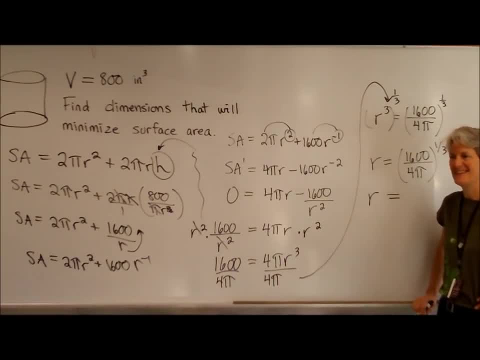 So we can figure out what r is equal to. What's your name? Tyra, Tyra, Hi, Tyra Tyra is going to calculate this for us in just a moment: 5.03.. Beautiful, We're rounding it to the nearest hundredth place. 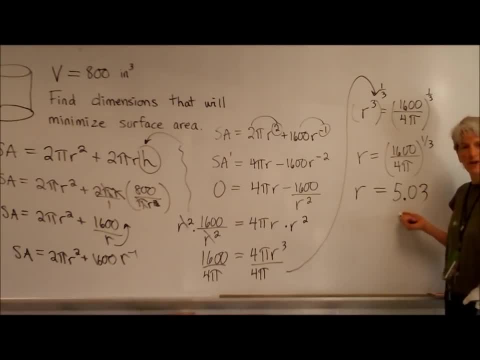 Thank you very much, Excellent. So if I wanted to, I could verify that this in fact is a minimum. You guys know how to do that. Set up your sign analysis, Make sure that in fact, it is a minimum. 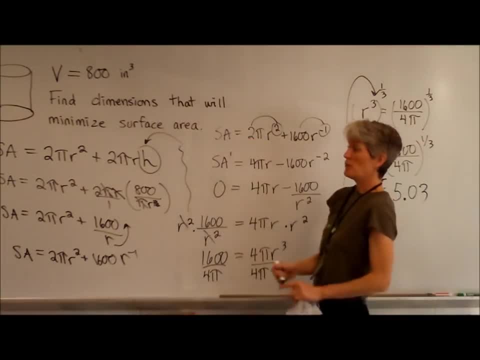 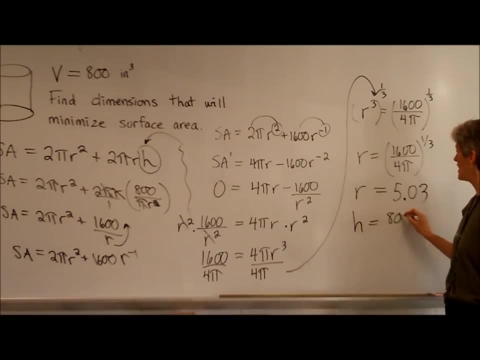 So let's skip that for now And let's go ahead and find what h is. I think I erased that, But if you remember, we had that hand equation that h was equal to 800.. Which was the volume divided by pi r squared. 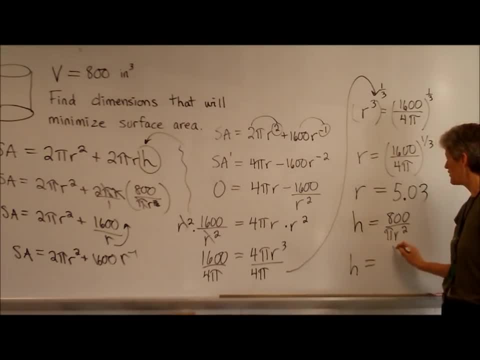 So I can take my radius And of course you're using your calculator back at home, So you would want to put the full- You know, the full- decimal in there, rather than the rounded version, to make sure you get an exact answer or as close to exact as possible. 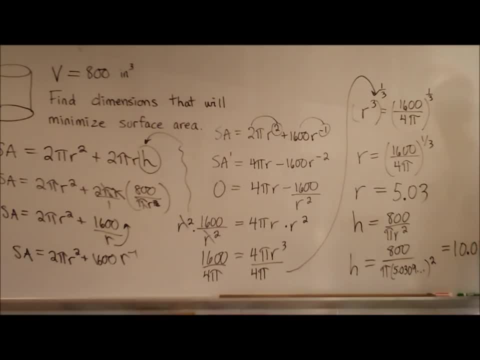 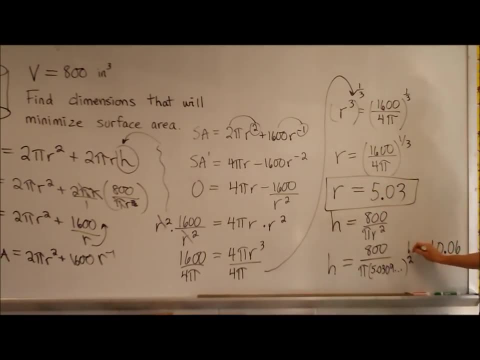 And you're going to end up with 10.06.. 10.06 inches. So my dimensions would be 5.03 inches by, for my radius and my height is 10.06 inches. And there you have it.